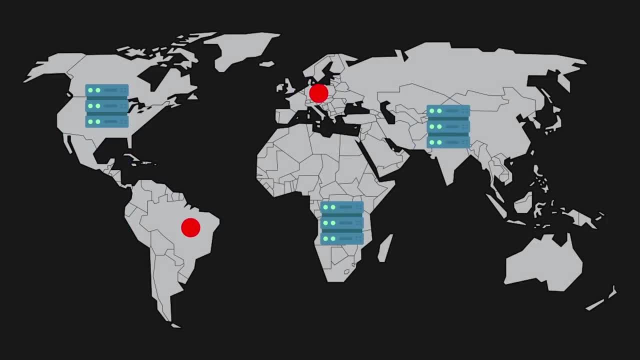 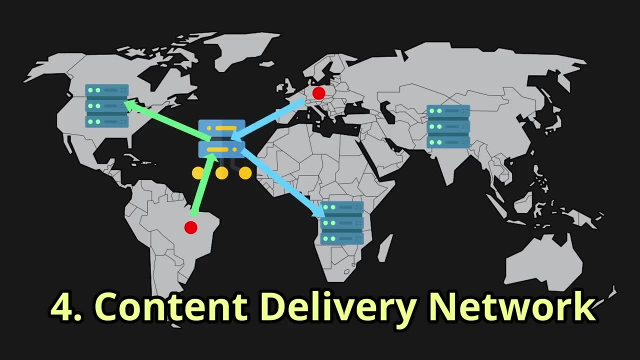 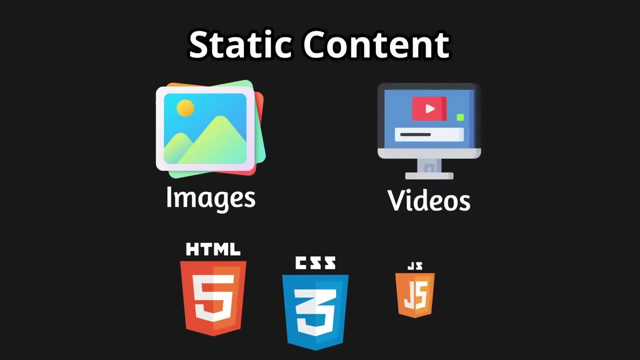 getting. But if our servers are located all around the world, we could even use a load balancer to route a request to the nearest location, Which brings us to content delivery networks. If you're using static files like images, videos and sometimes even HTML, CSS and JavaScript files, 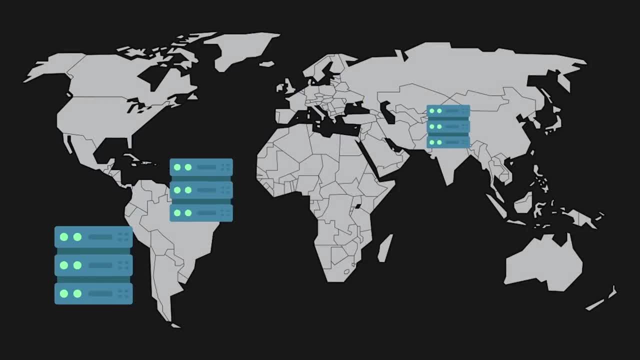 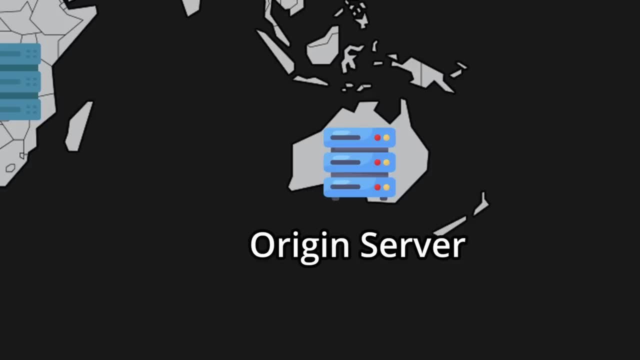 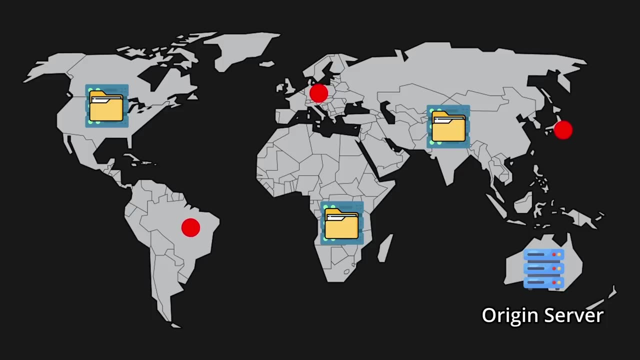 you can just use a CDN. It's a network of servers located all around the world. CDNs don't really run any application logic. They work by taking files hosted on your server, aka the origin server, and copying them onto the CDN servers. This can be done either on a push. 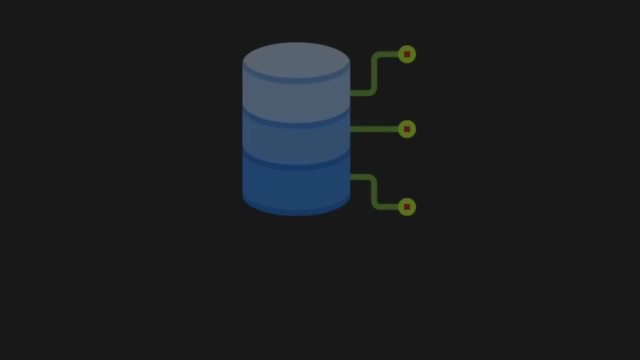 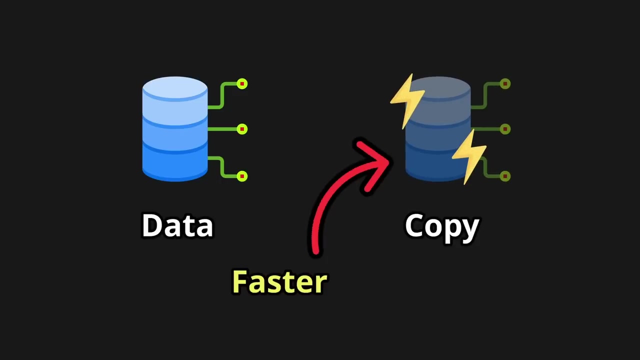 or pull basis. But CDNs are just one technique. So let's take a look at some of the things that can be done with CDNs. First off, we have the ability to cache. CDNs are a very unique tool for caching. 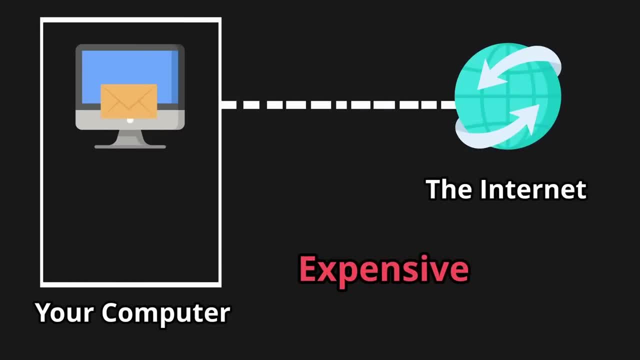 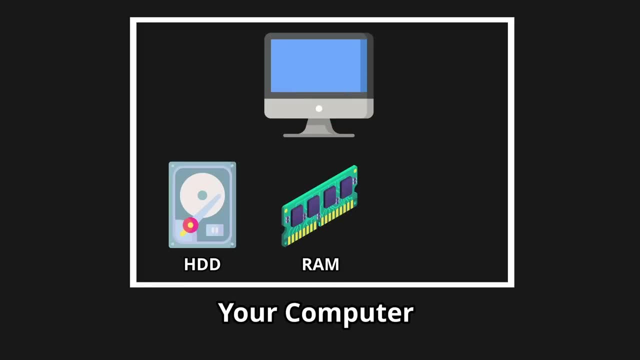 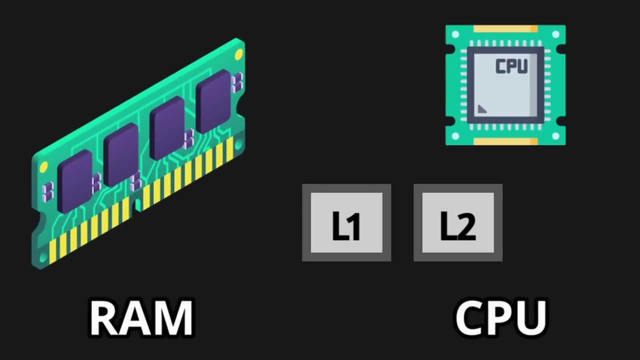 which is all about creating copies of data so that it can be refetched faster in the future. Making network requests can be expensive, so our browsers will sometimes cache data onto our disk. But reading disk can be expensive, so our computers will copy it into memory, But reading memory can. 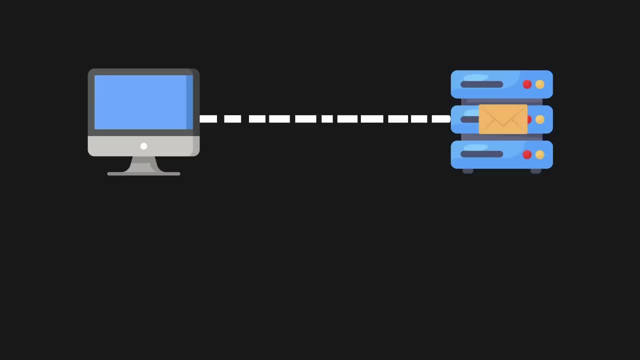 be expensive, so our operating systems will copy a subset of it into our L1,, L2, or L3 CPU cache. So how do computers communicate with each other? Well, every computer is assigned an IP address which uniquely identifies a device on a network. And to round it all out, we have the poorly named 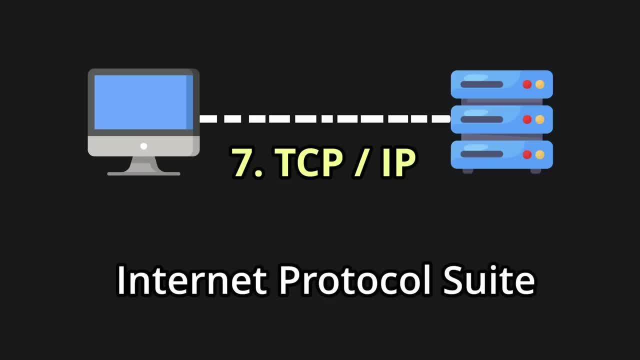 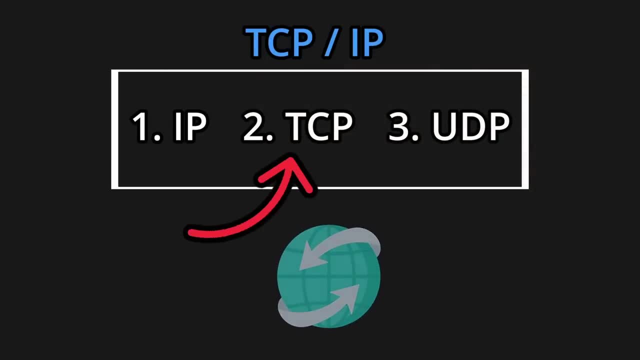 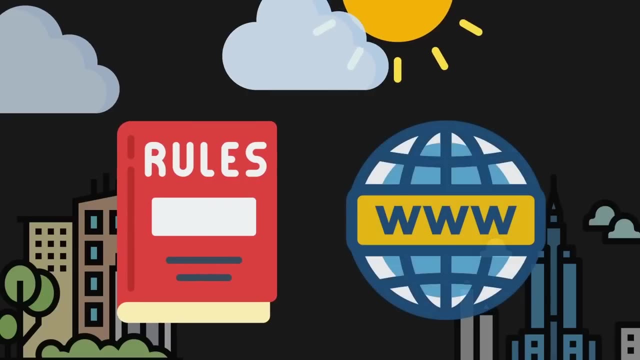 TCP, slash, IP or the Internet Protocol Suite, since it actually includes UDP as well. But focusing on TCP for a second, there has to be some set of rules aka protocols that decide how we send data over the internet, Just like how, in real life, we have a system that decides how we send mail to each other. 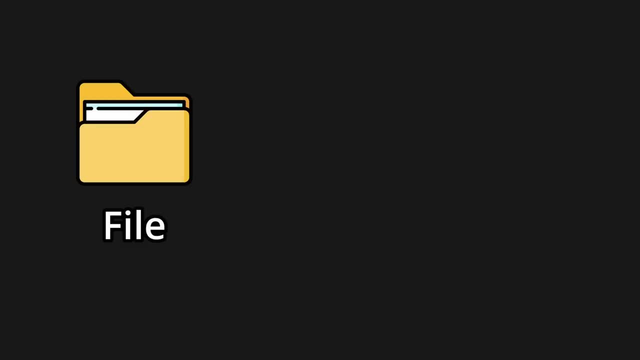 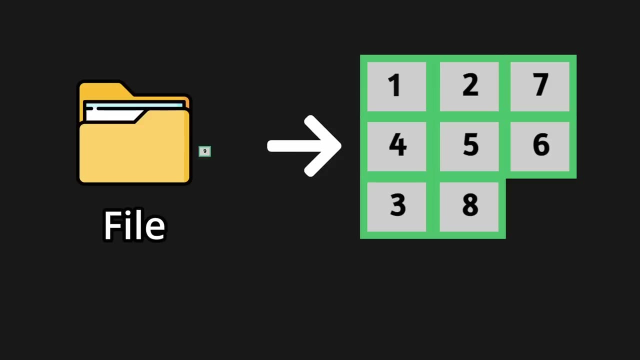 Usually, when we send data like files, they're broken down into individual packets and they're sent over the internet, And when they arrive at the destination, the packets are numbered so that they can be reassembled in the same order. If some packets are missing, TCP ensures that they'll be re-sent. 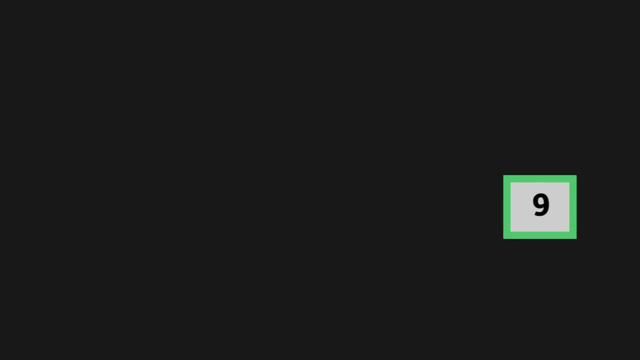 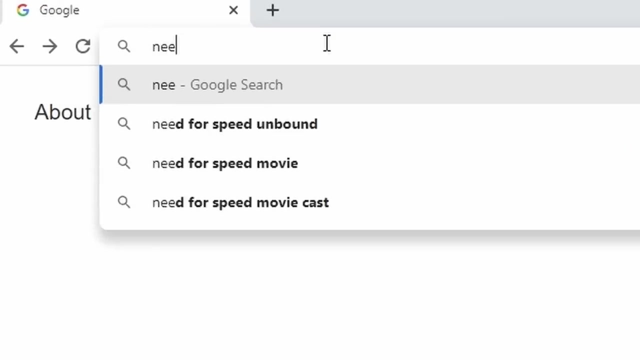 This is what makes it a reliable protocol and why many other protocols like HTTP and WebSockets are built on top of TCP. But when you type neatcodeio into your search bar, how does your computer know which IP address it belongs to? 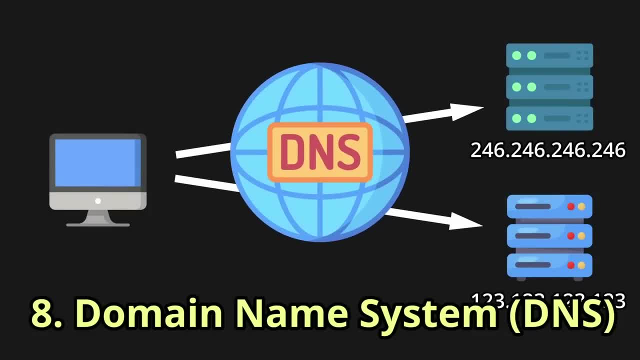 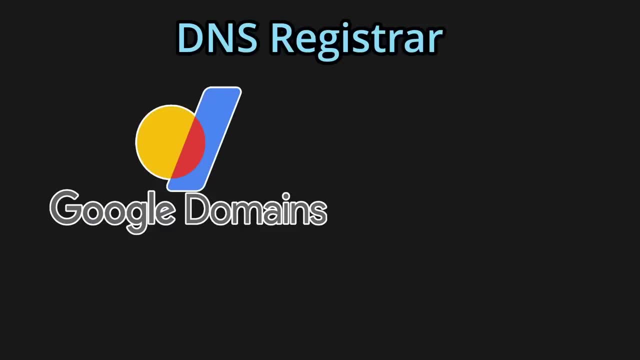 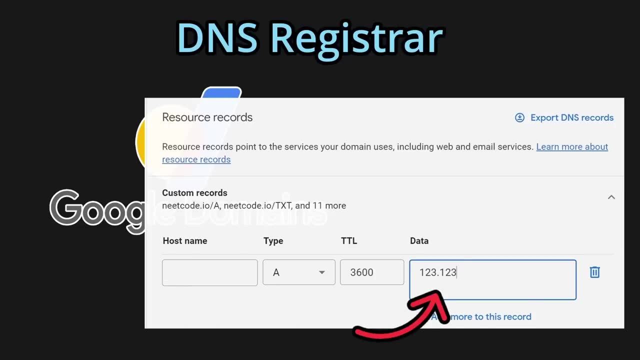 Well, for that we have the domain name system, which is a largely decentralized service that works to translate a domain to its IP address. When you buy a domain from a DNS registrar, you can create a DNS-A record, which stands for address, and then you can enter the IP address of. 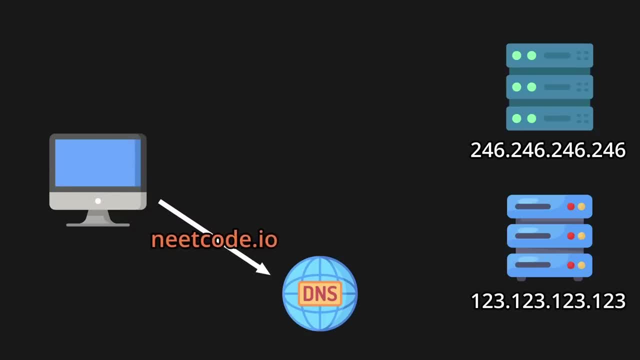 your server. So then, when you search and your computer makes a DNS query to get the IP address, it'll use the A record mapping to get the address and then your operating system will cache it so that it doesn't need to make a DNS query every single time. 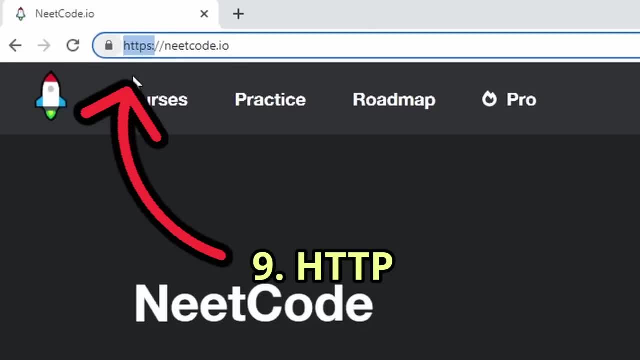 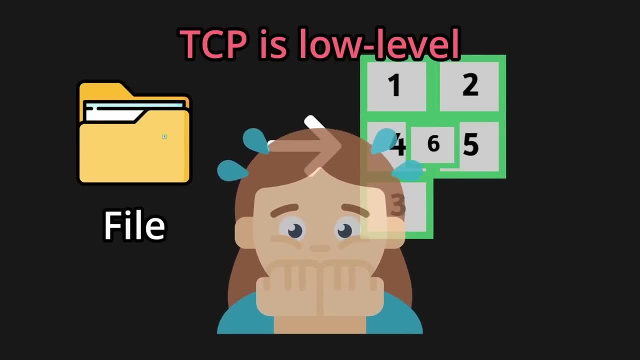 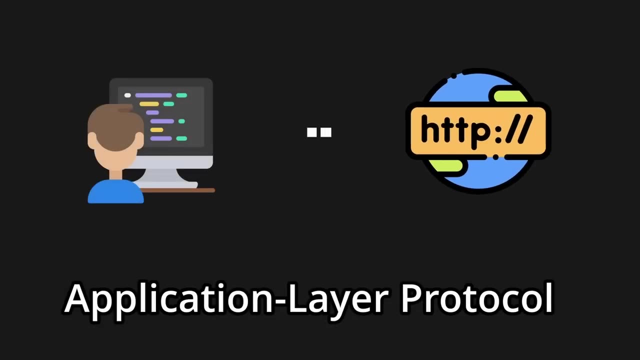 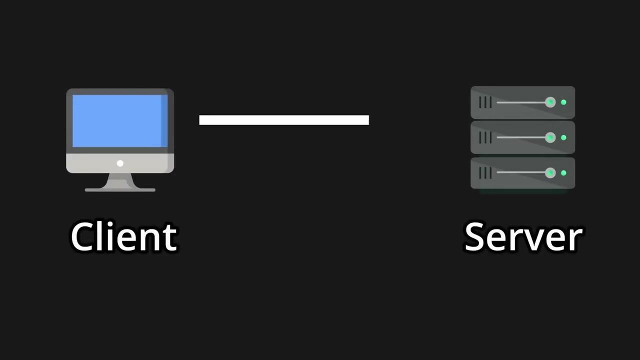 But wait a minute. why do we usually use HTTP to view websites? Well, TCP is too low level. We don't want to have to worry about individual data packets, so we have an application-level protocol like HTTP. HTTP follows the client-server model where a client will initiate a request. 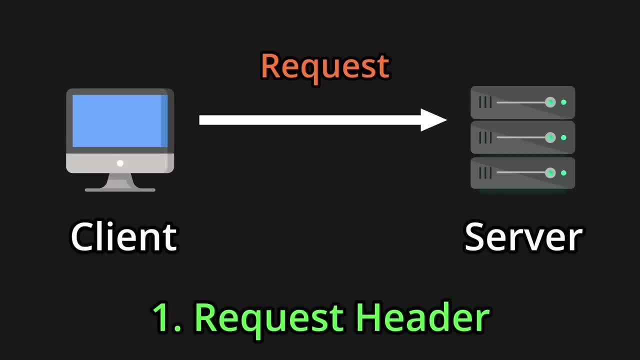 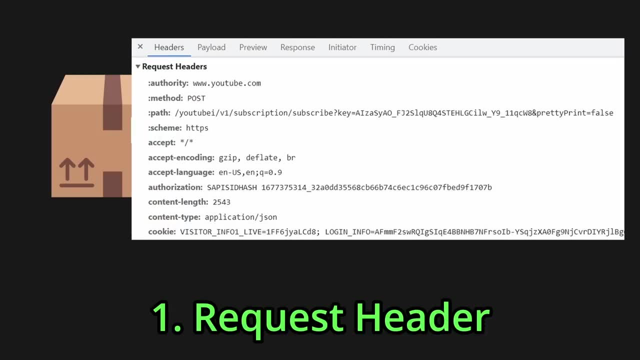 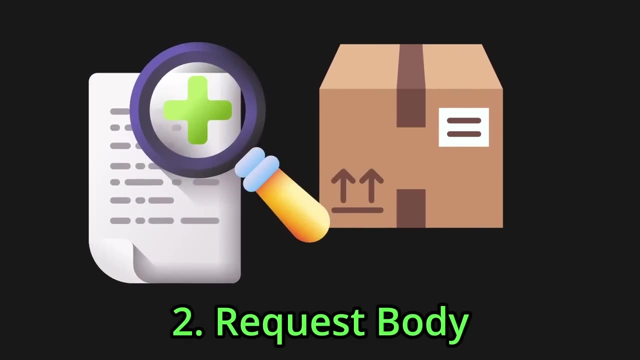 which includes two parts. One, the request header. Think of that as the shipping label you put on a package. It tells you where the package is going, who it's from and maybe some other metadata about the package itself. The second part is the request body, which is basically the package contents To. 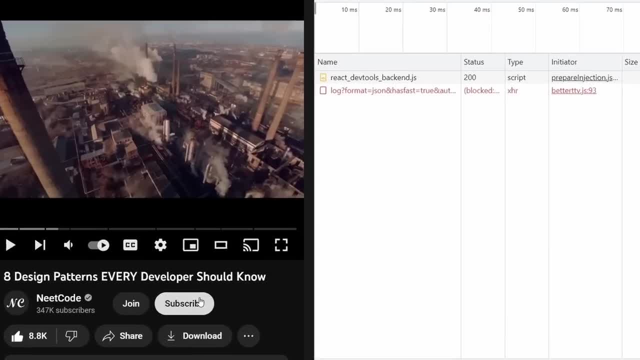 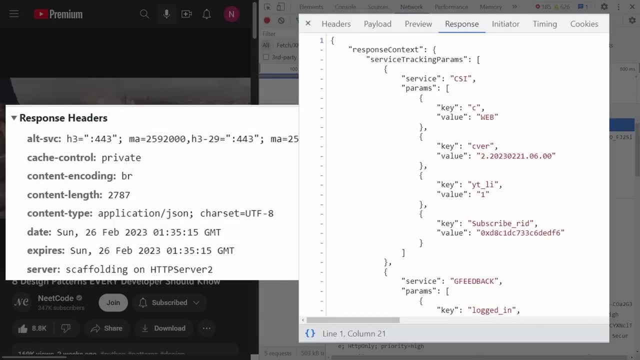 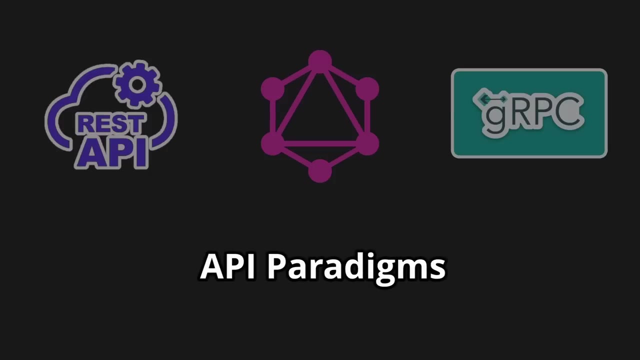 test it out. just open your DevTools network tab and click subscribe. Go on, I'll wait. Taking a closer look at the request, we can see that the response also includes a header as well as a body. But even with HTTP, there are multiple API patterns we could follow. 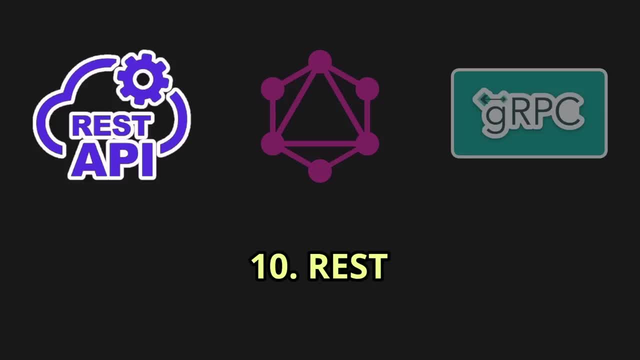 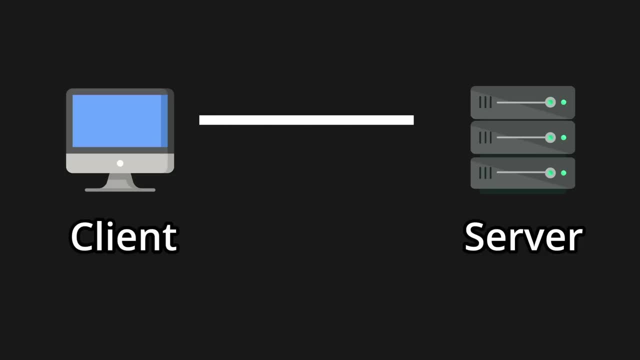 the most popular one being REST, which is a standardization around HTTP APIs, making them stateless and following consistent guidelines. Like a successful request should include the following: Your API is 100 times faster. your page is 100 times faster. your. 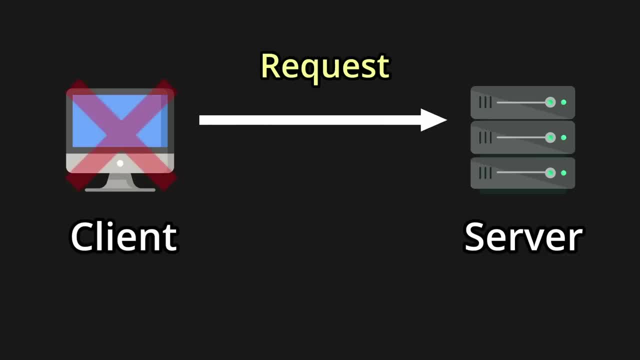 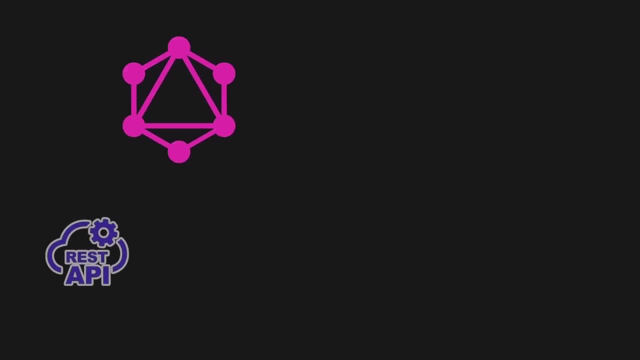 code in its response header, whereas a bad request from the client would return a 400 code and an issue with the server would result in a 500 level code. GraphQL is another API pattern introduced by Facebook in 2015.. The idea is that, instead of making another request for every single 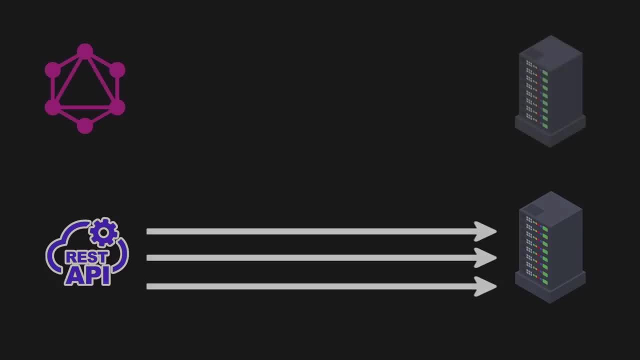 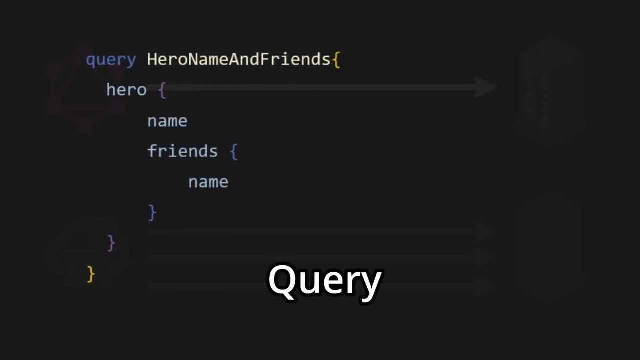 resource on your server, like you would do with REST. with GraphQL, you can just make a single request, aka a query, and you can choose exactly which resources you want to fetch. This means you can fetch multiple resources with a single request and you also don't end up over-fetching. 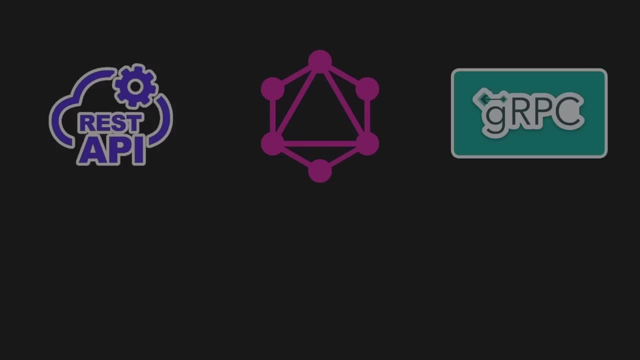 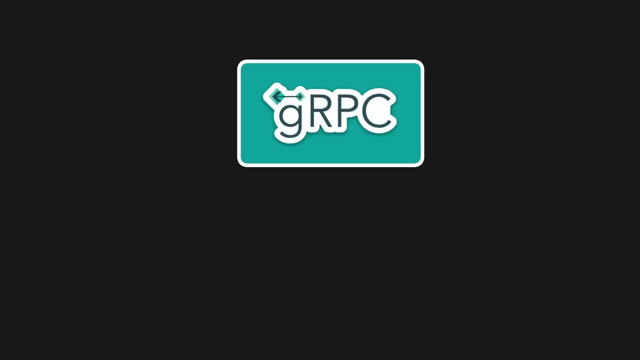 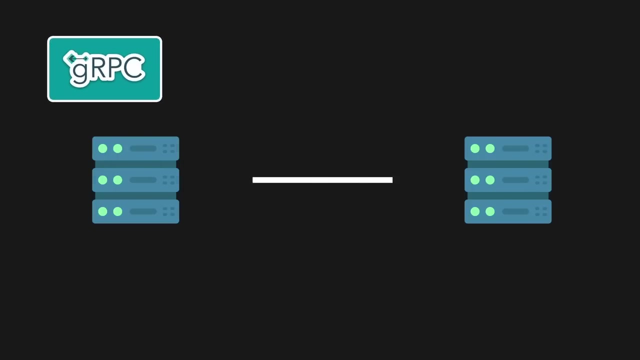 any data that's not actually needed. Another API pattern is gRPC, though it's really considered a framework Released by Google in 2016,. it was also meant to be an improvement over REST APIs. It's an RPC framework mainly used for server-to-server communication. 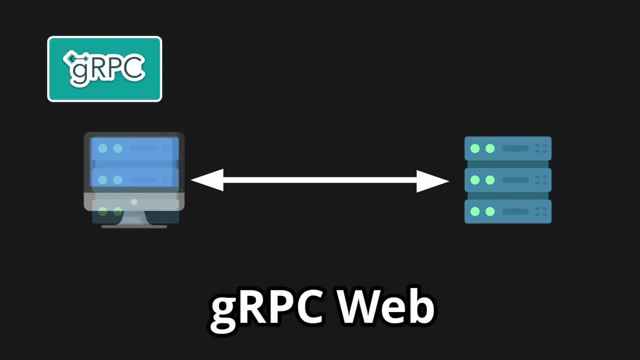 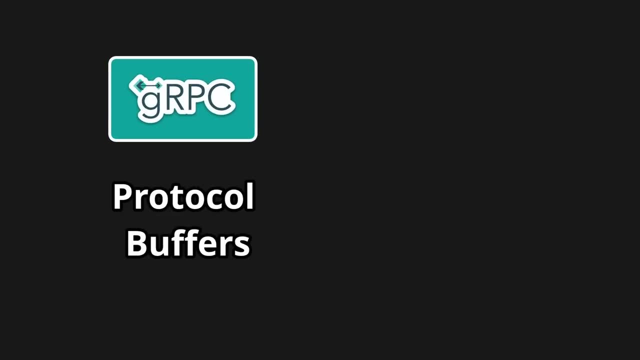 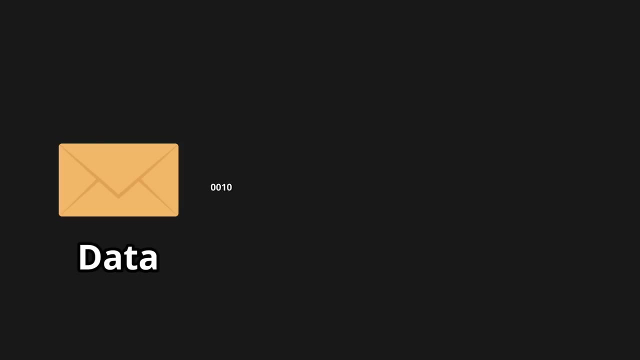 but there's also gRPC Web, which allows using gRPC from a browser which has also been growing quickly over the last few years. The performance boost comes from protocol buffers, Comparing them to JSON, which is what REST APIs use. protocol buffers are an improvement in that data is. 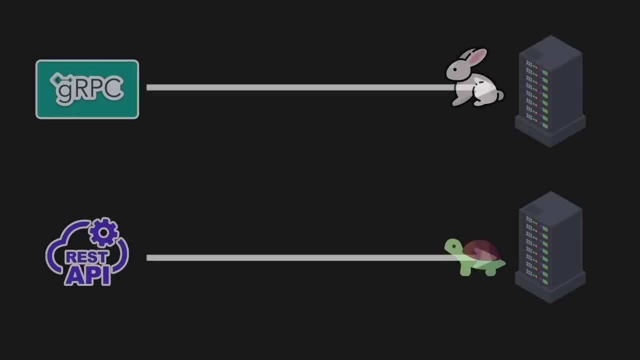 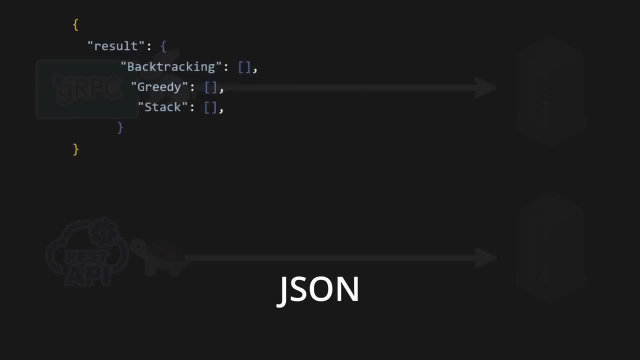 serialized into a binary format, which is usually more storage efficient and, of course, sending less data over a network will usually be faster. The downside is that JSON is a lot more human-readable, since it's just a data-driven system. So if you're using a data-driven system, you can use a. 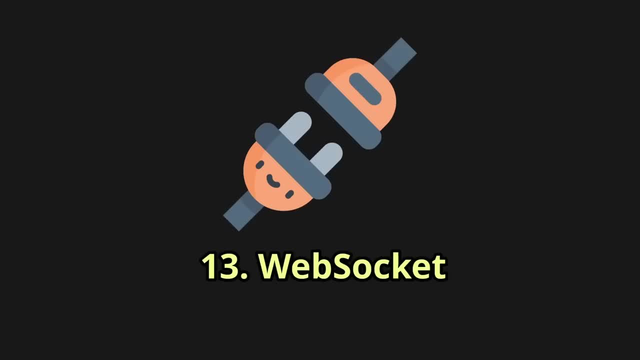 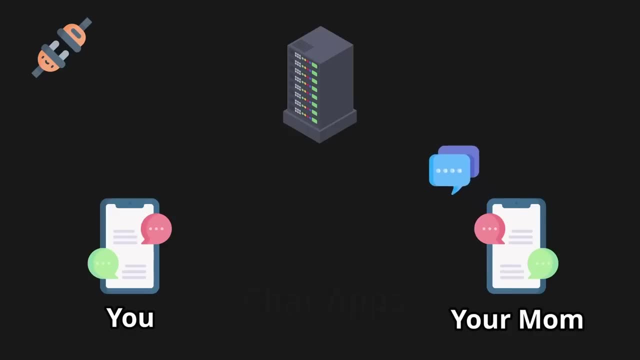 plain text. Another app layer protocol is WebSockets. To understand the main problem that it solves, let's take chat apps, for example. Usually, when someone sends you a message, you receive it immediately. If we were to implement this with HTTP, we would have to use polling. 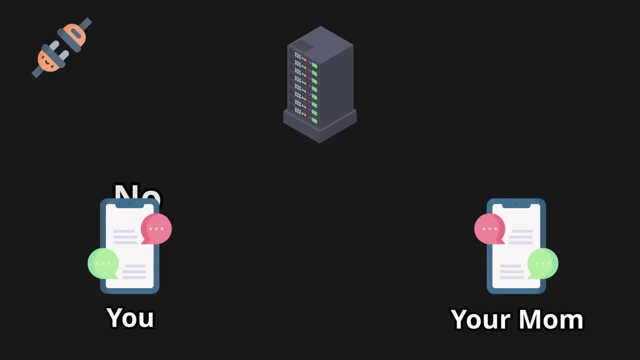 where we would periodically make a request to check if there was a new message available for us. But unlike HTTP1, WebSockets support bi-directional communication, So when you get a new message, it's immediately pushed to your device, And whenever you send a message, it's immediately. 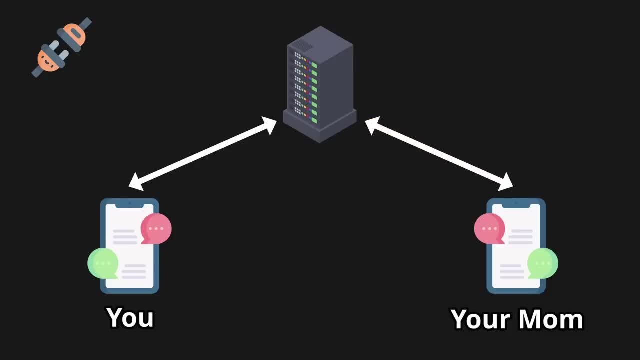 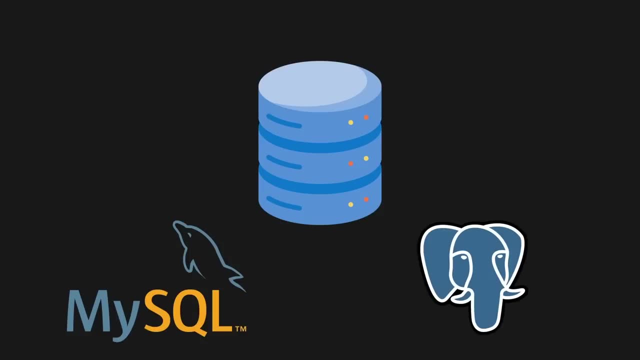 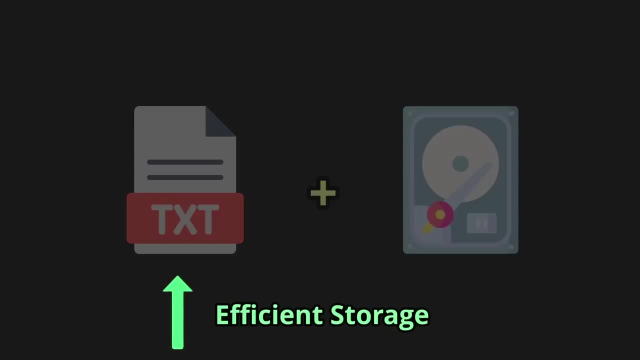 pushed to the receiver's device. And for actually storing data we have SQL or relational database management systems like MySQL and Postgres. But why should we use a database when we can just store everything in text files stored on disk? Well, with databases we can more efficiently. 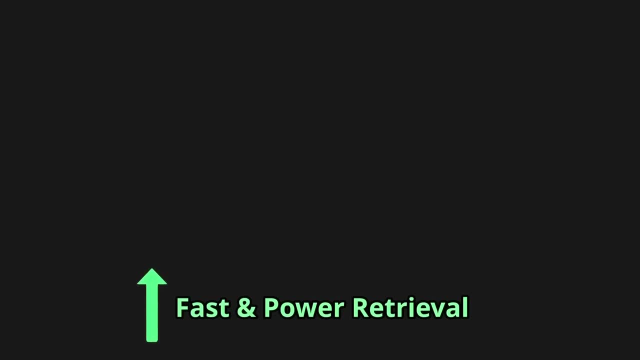 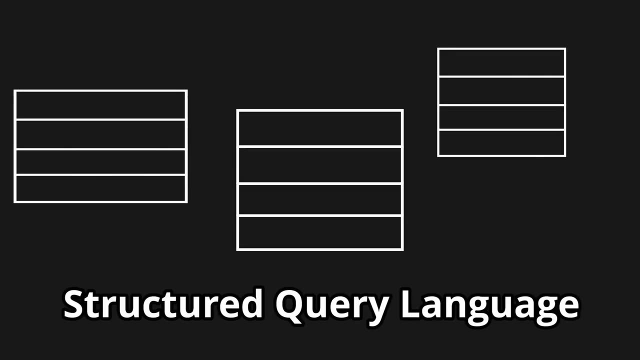 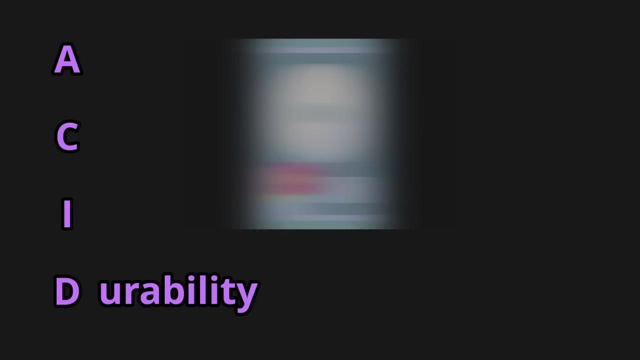 store data using data structures like B-trees, and we have fast retrieval of data using SQL queries, Since data is organized into rows and tables, Relational database management systems are usually ACID compliant, which means that they offer durability because data is stored on disk. 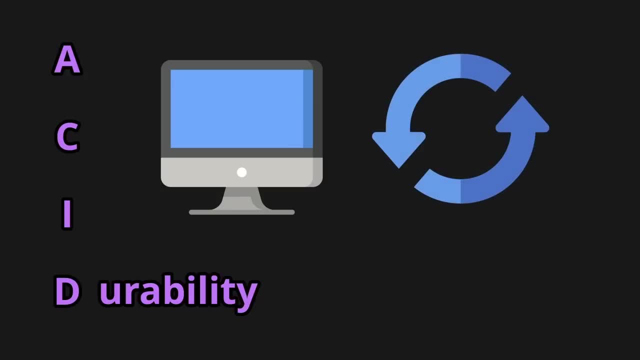 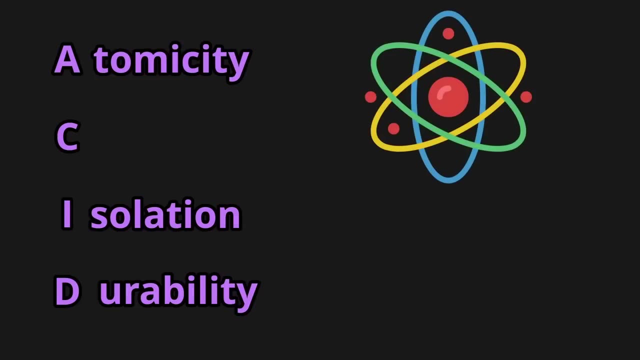 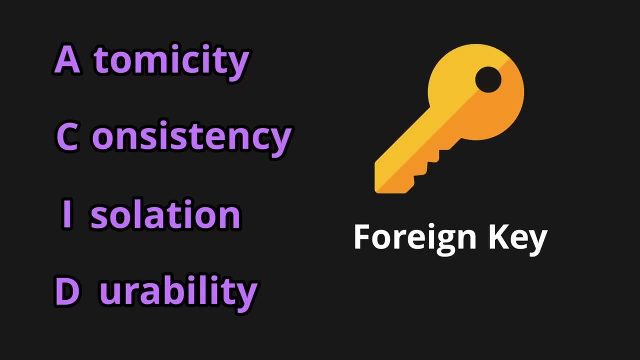 So, even if a machine restarts, the data will still be there. Isolation means that different concurrent transactions won't interfere with each other. Atomicity means that every transaction is all or nothing. Lastly, we have consistency, which means that foreign key 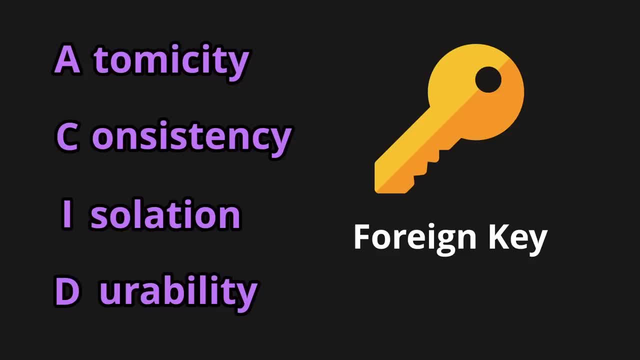 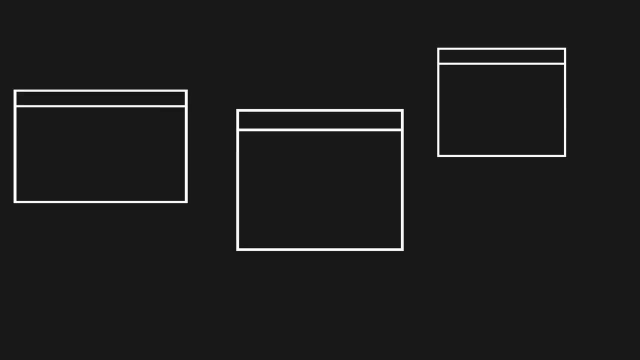 and other constraints will always be enforced. This one is really important because it led to the creation of NoSQL, or non-relational databases. Consistency makes databases harder to scale, So NoSQL databases drop this constraint and the whole idea of relations altogether. 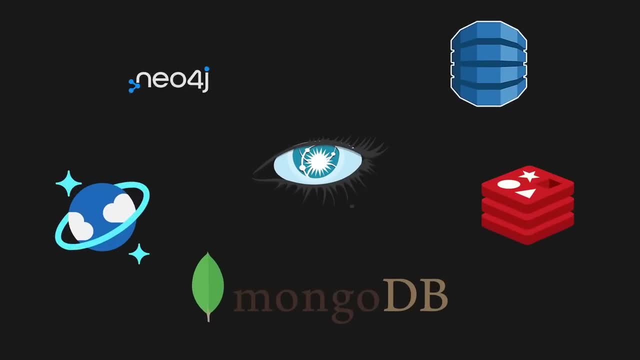 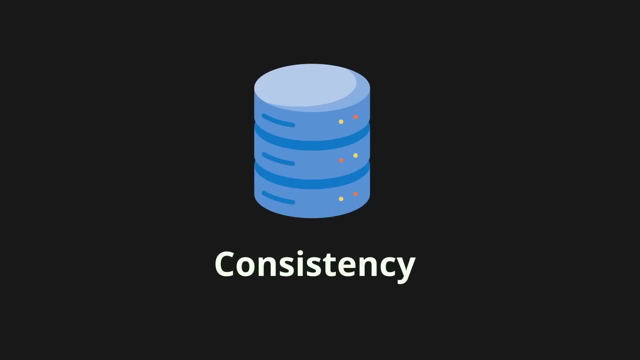 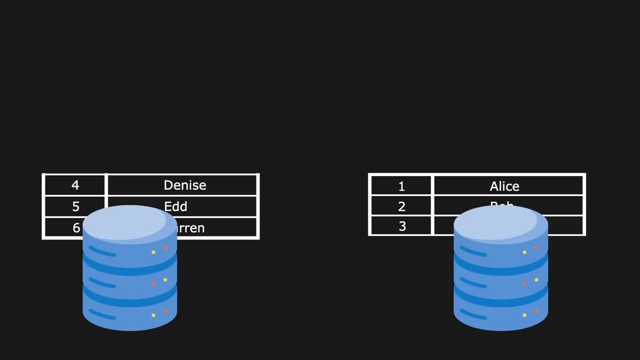 There are many types of NoSQL databases, but popular ones include key value stores, document stores and graph databases. But going back to consistency, if we don't have to enforce any foreign key constraints, that means we can break up our database and scale it horizontally with different machines. This technique is called sharding. 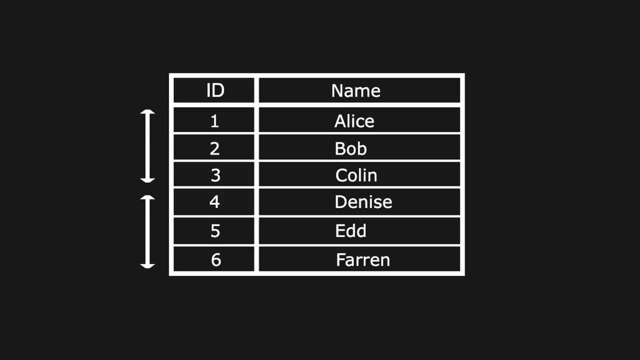 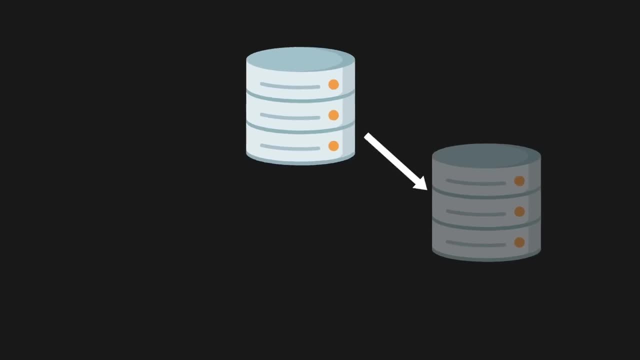 But how do we decide which portion of the data to put on which machine? Well, for that we usually have a shard key. So, given a table of people, our shard key could be the ID of the person. But sharding can get complicated. A simpler approach is replication. If we want to scale our 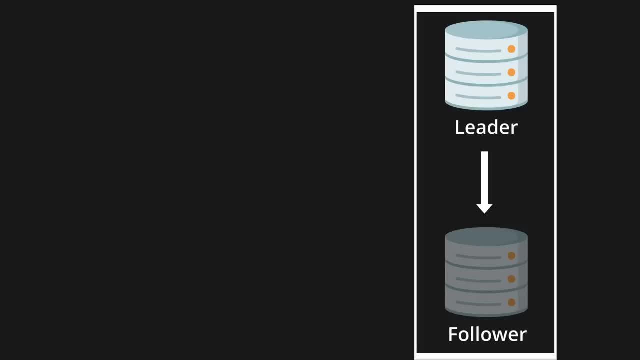 database reads. we can make read-only copies of our database. This is called leader-follower replication, where every write will get sent to the leader, who sends those to the followers, but every read could go to a leader or a follower. There's also leader-leader replication. 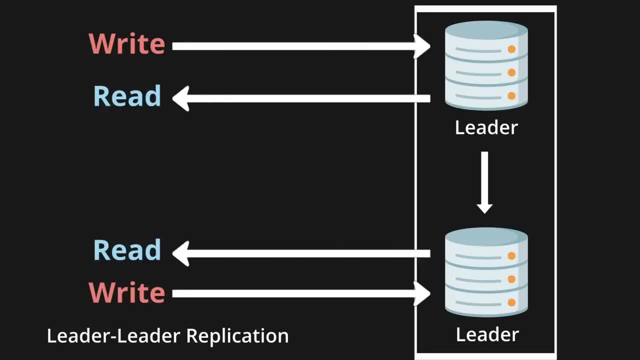 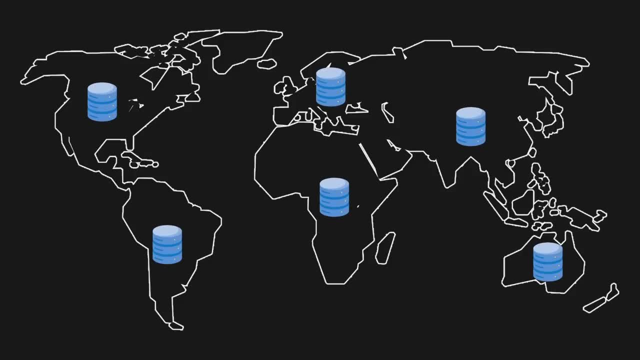 where every replica can be used to read or write, but this can result in inconsistent data, so it would be best to use it where you can have a replica for every region in the world, for example. It can be complex, but it's not a problem. So let's take a look at some of the 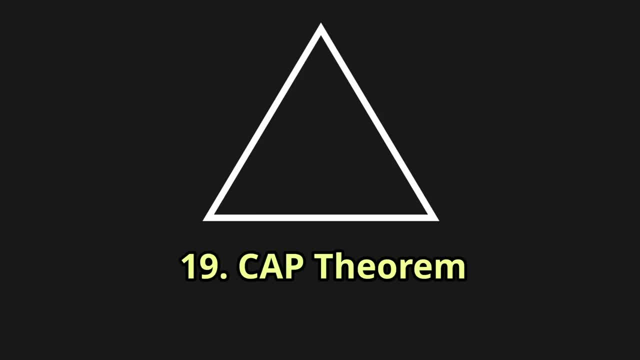 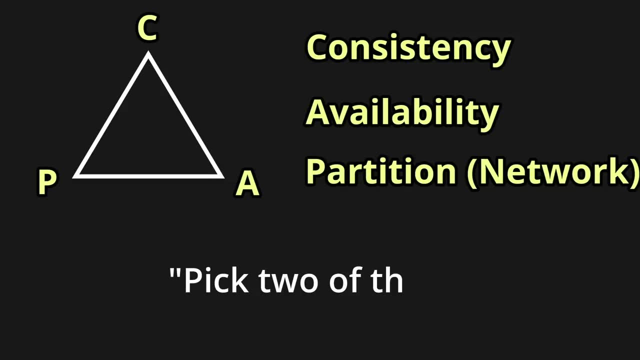 to keep replicas in sync. So the CAP theorem was created to weigh trade-offs with replicated design. It states that, given a network partition in a database, as database designers we can only choose to favor either data consistency or data availability. What makes it confusing is that 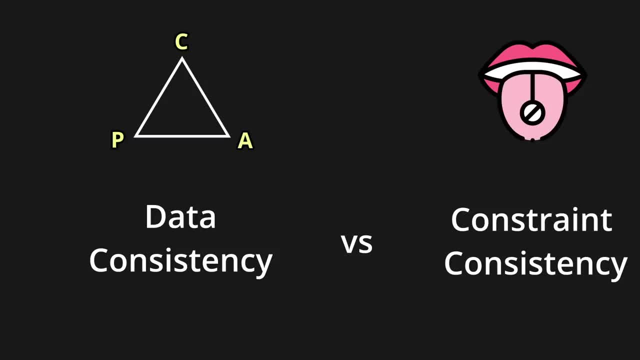 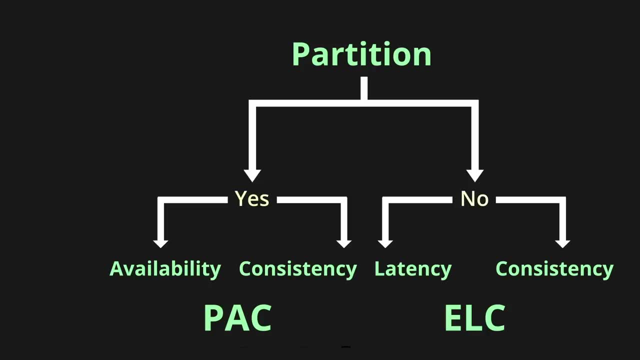 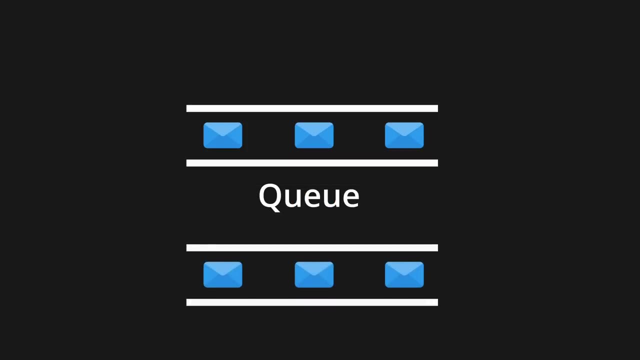 consistency here means something different than with ACID. It's a somewhat controversial theorem, which is why the more complete PAC-ELSE theorem was created. Lastly, we have message queues. They're kind of like databases because they have durable storage and they can be replicated for redundancy or sharded for scalability. but they have many.